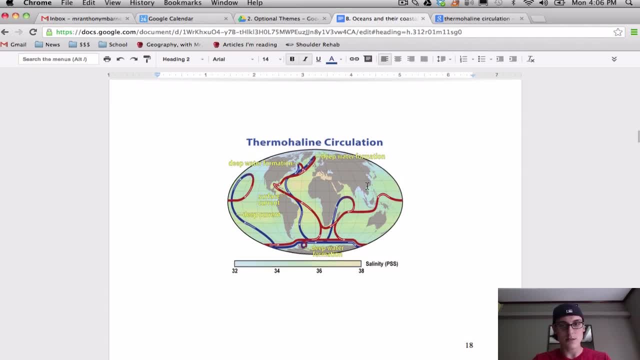 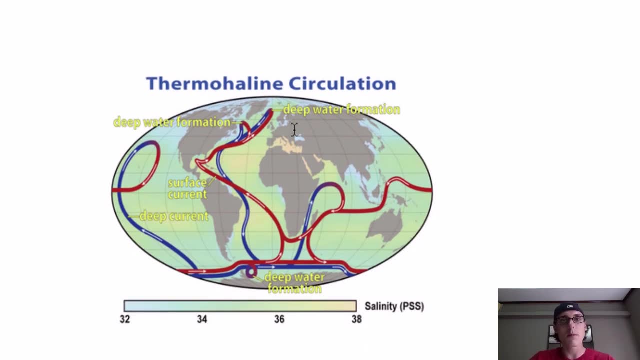 get to this map, alright. So let's take a look at this map and what this map actually means: The thermohaline circulation. there's two main important things that you're going to want to remember, okay, The first one is this title: thermohaline- alright. 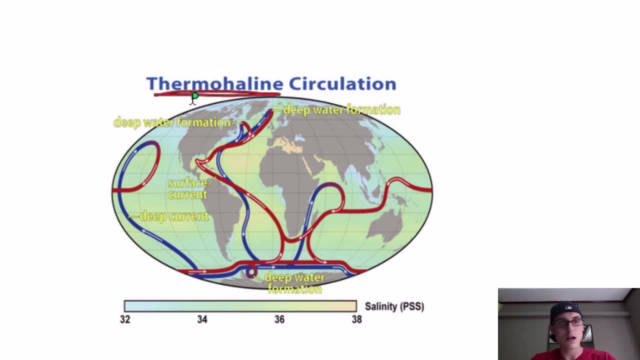 You can break this up into two separate words: Thermo, meaning temperature, and haline, meaning salinity or salt. alright, The reason that it's called the thermohaline circulation or temperature salt circulation is simply because the ocean water is driven on the surface by wind. 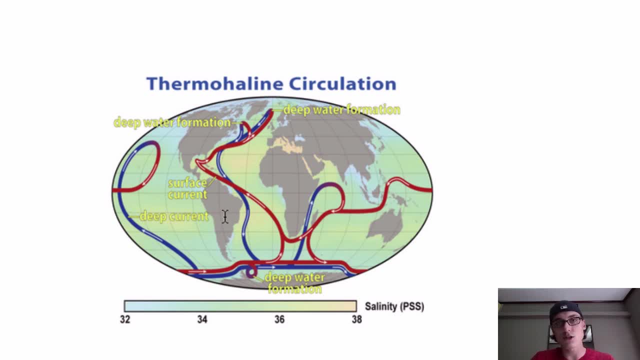 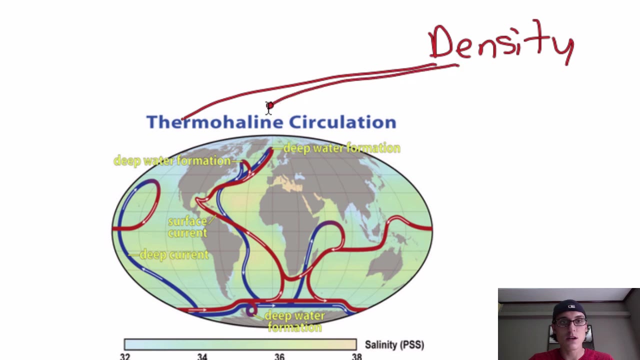 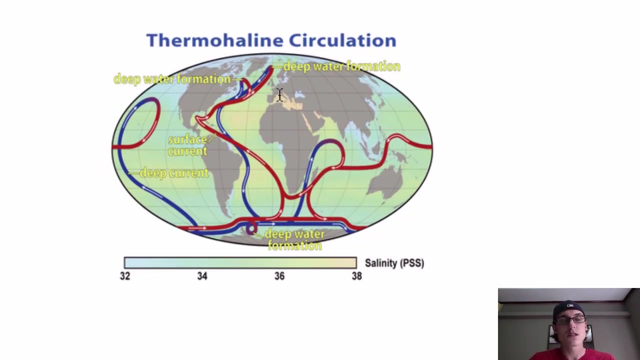 is driven through the depths of the ocean by the temperature and salinity. We also say that the density of the ocean water is dependent on the temperature and the salinity. So, if you can remember from physics class, cold, salty water will sink more readily than warm. 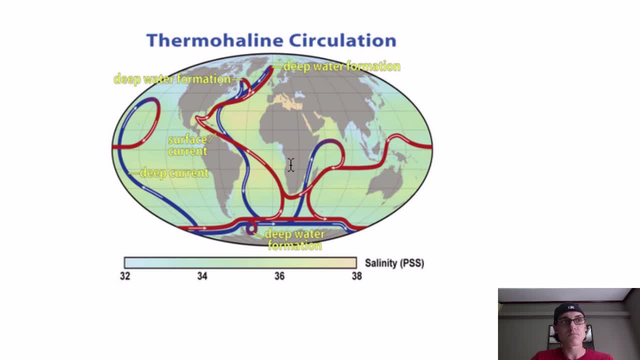 clear water, and so, um, the, the cold water is more dense, and because it has more salt in it, that causes it to be more dense, and so, um, that's the, the main idea with the, the name itself, thermohaline circulation, so the, um, the density gradient is what drives the deep water through. 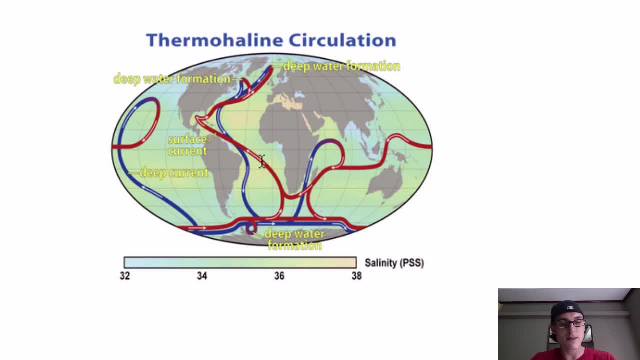 its ocean basins. now, before i get too far ahead of myself, let me just describe what's happening, what you have on the surface, if is you have uh winds blowing that surface water, all right, in the northern hemisphere, in this direction, and in the southern hemisphere, in 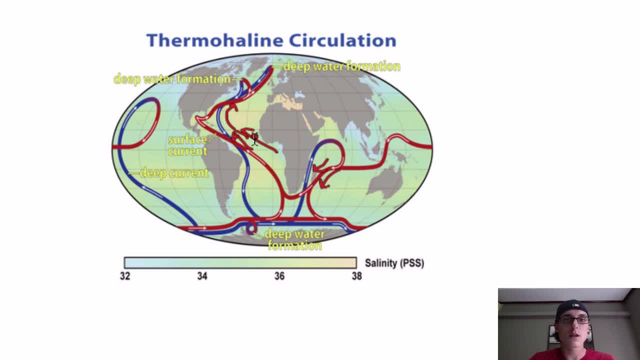 this direction. okay, so warm waters are blown by- uh, by wind along the surface where they get too close to the poles, all the while becoming saltier and saltier until they reach the poles, in which case they actually sink down into the depths of the ocean. and the reason they sink again is because 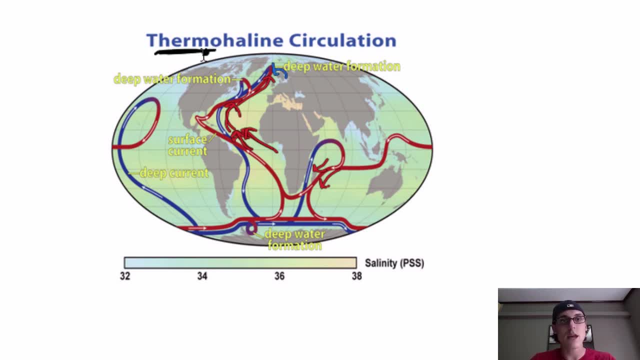 of that thermal helium engine. they call it even the the great ocean conveyor, and it's the, the salt and the, the temperature of the water, that drives this, this conveyor. so you have again the warm surface currents moving along the equator and up into the poles where the water becomes dense. 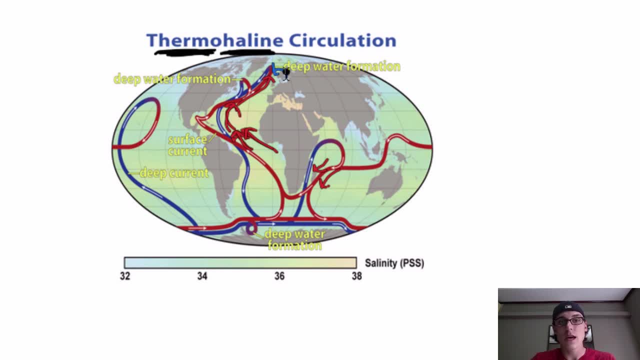 because it is too salty and cold, and so it drops down into the depths of the ocean, where it's then driven along ocean basins, as this water up on the surface, you know, piles of water drop down into the ocean and then it becomes dense and so it becomes too salty and 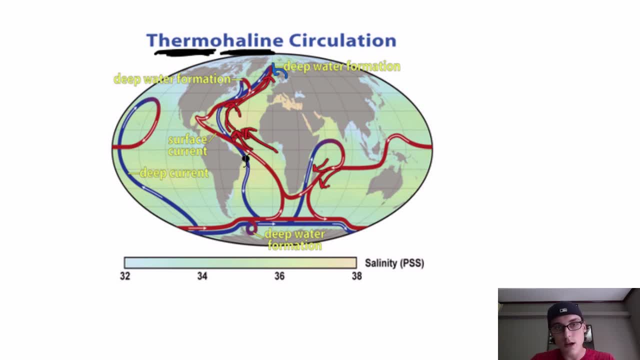 you know, piles of water, and then it becomes super salty, and then it becomes too salty and so it impacts up behind it. it drives that that deep water along the ocean basins where it will finally up, well, in the, the southern ocean typically, or it might, you know, do a whole loop around this Antarctic. 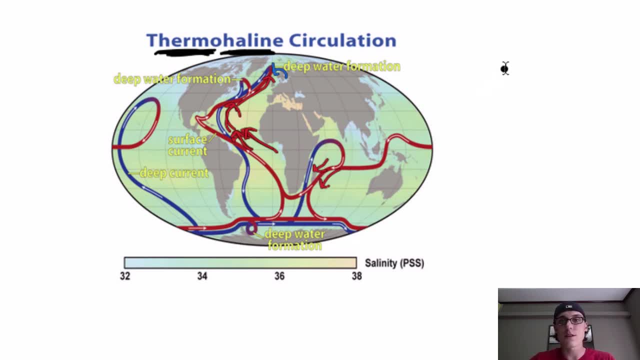 continent, where then it will finally up? well, the, the total time is estimated to be 1,000 to 1,500 years for the one, let's say one water molecule to make its way around the entire, you know, circulation of the planet. alright, so that's, that's the one first main thing, so that's the 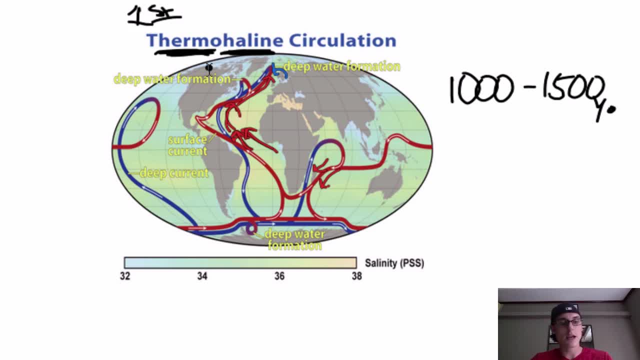 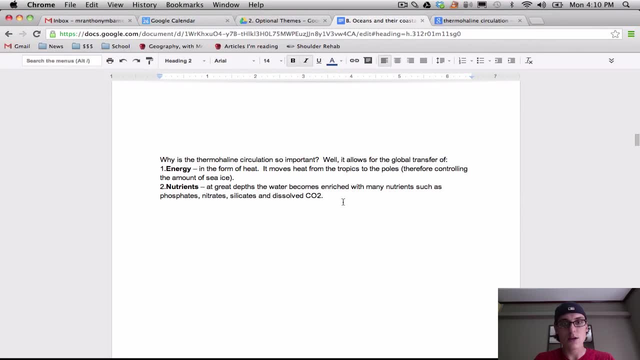 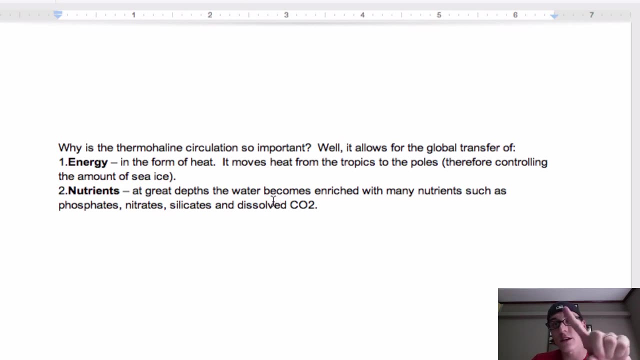 first first main idea. okay, the second main idea is what you'll find a little bit lower on your Google Doc. you'll see it here. the second main idea is why. the third main idea is why the thermohaline circulation is important. So the first thing that you need to know is you need 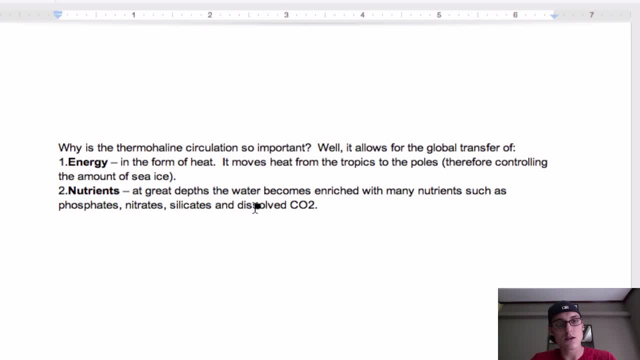 to know how it operates. And then the second thing you need to know- this is your second main idea, okay. Your second point is why it's important that the thermohaline circulation occurs in the first place. anyways, all right. The main two reasons is because it regulates the climate. 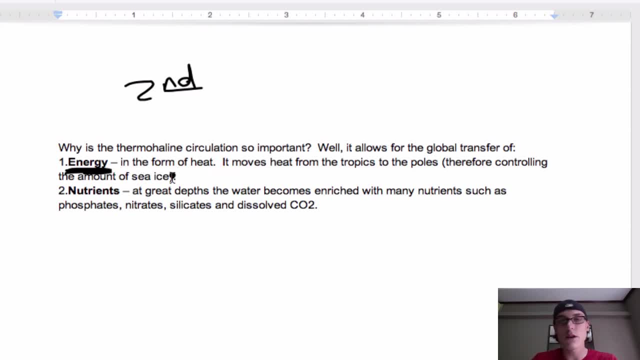 So in the form of heat. it transfers heat around the planet and that essentially regulates the climate. It keeps the certain areas of the planet either warmer or cooler, so that we have a proper regulation of the climate. It also another thing it does is it determines how much sea ice is in.